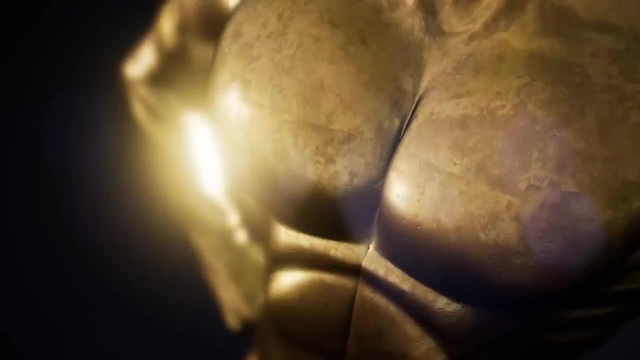 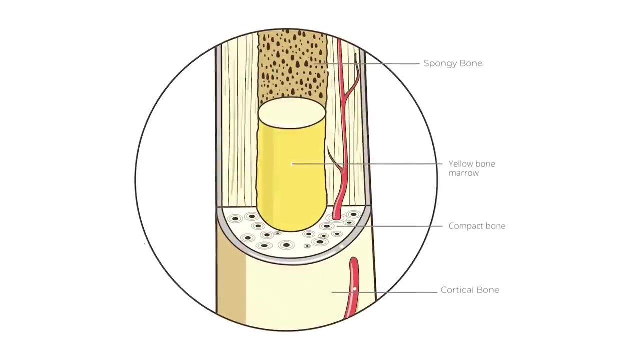 Spongy does not mean that these bones aren't strong. They are very strong and made to endure all the active things you do like running, jumping and playing. responsive bone marrow is in the holes of your spongy bones. Bone marrow has cells. 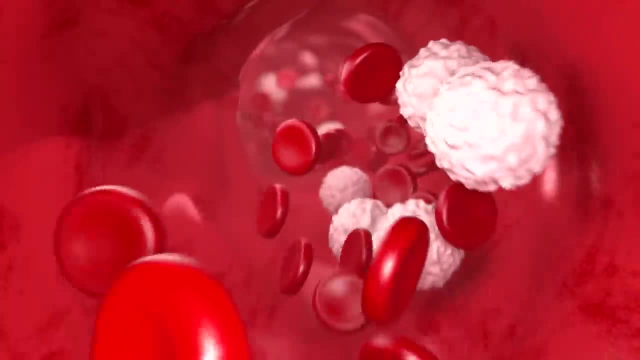 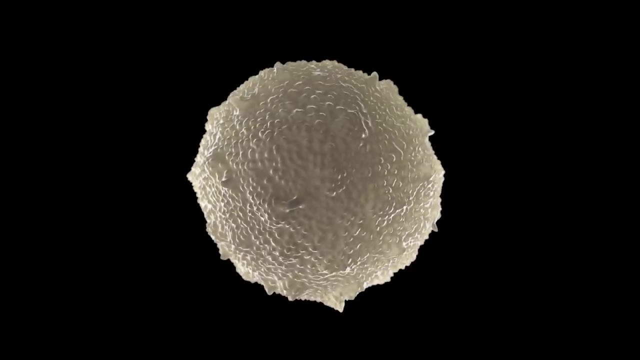 in it, called stem cells, which develop into red blood cells and white blood cells. Red blood cells carry oxygen throughout your body, while white blood cells fight infections in your body and help you get better. There are also platelets in your bone marrow. These 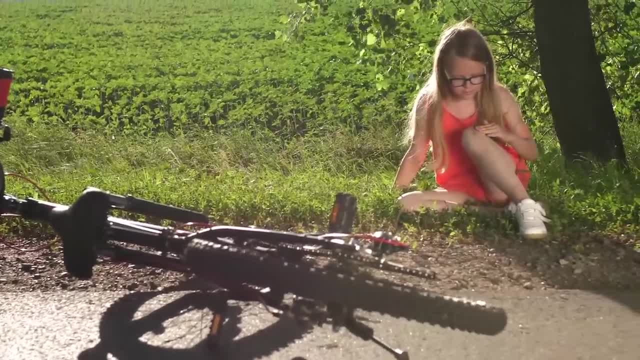 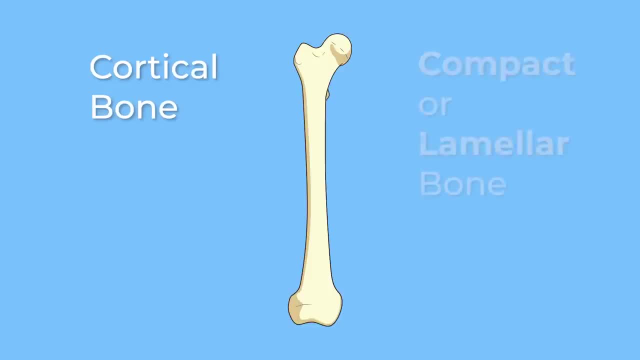 help with blood clotting. If you get cut, they cause your blood to form a scab and stop bleeding. Cortical bones are the other types of bone bones in your body. They are also called compact or lamellar bones. Cortical bones are made up of: 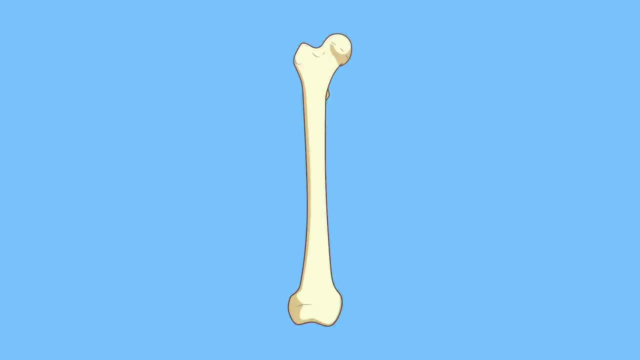 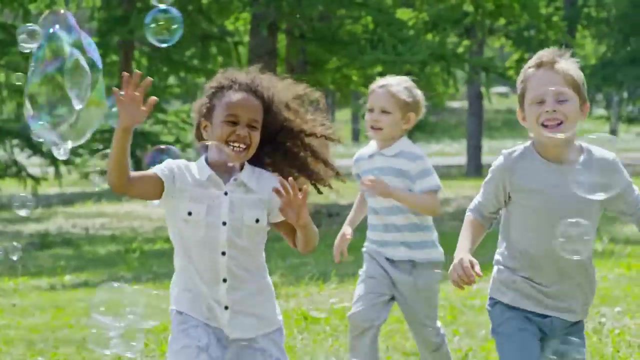 a thicker and stiffer material, They are very strong. Cortical bones make up 80% of your skeleton. These bones give strength to your longer bones. The different types of bones in your body have different jobs to do. Long bones, like the ones in your arms and legs, are there to support. 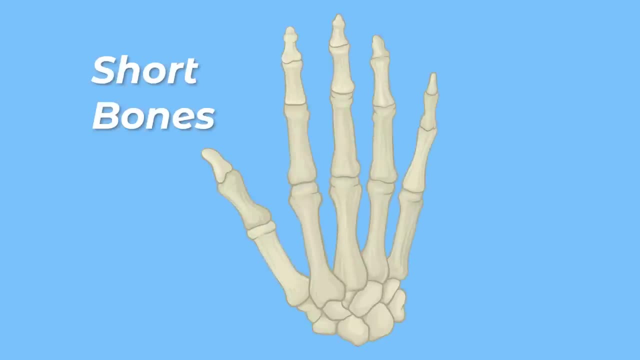 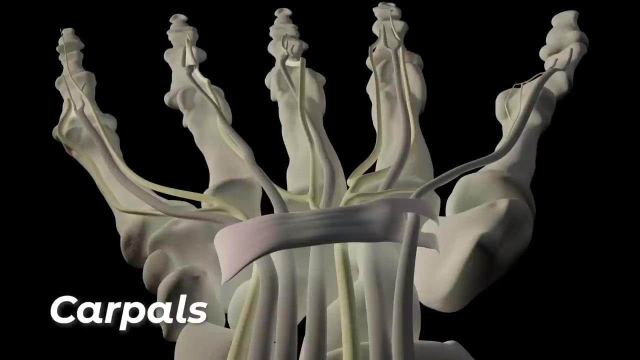 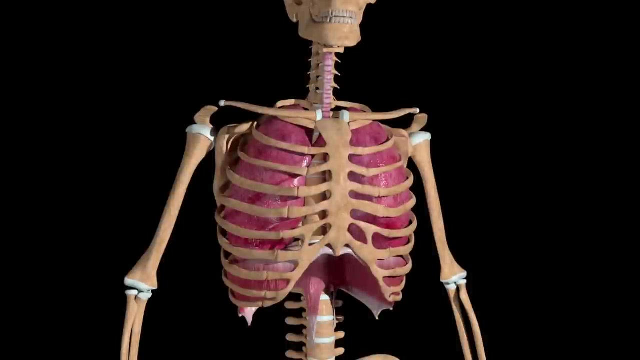 the weight of your body. Your body also has bones called short bones. These bones look like little cubes and are in your wrists, called carpals, and your feet, called tarsals. There are also flat bones like your forehead or skull. Your sternum and ribs are flat bones too. They are located. 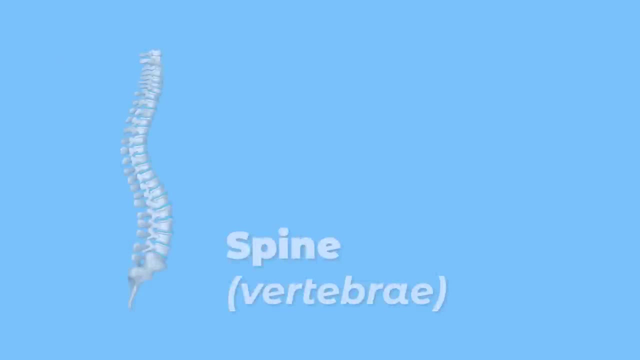 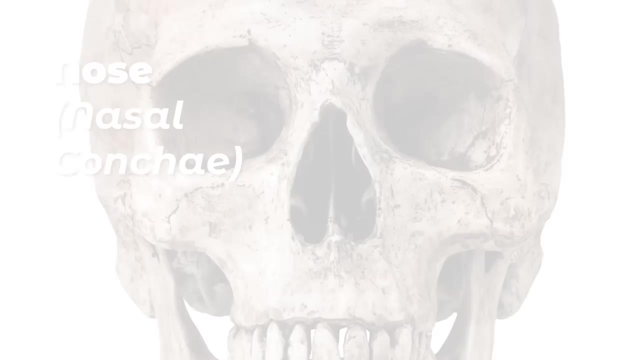 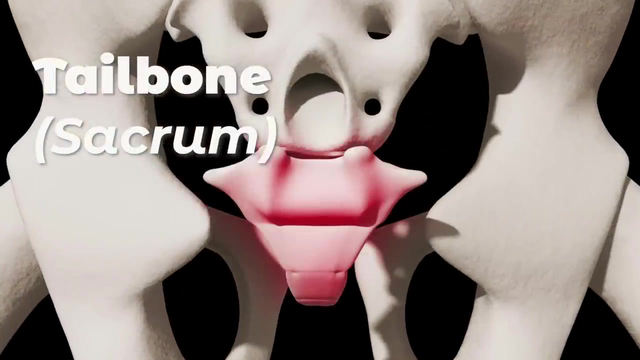 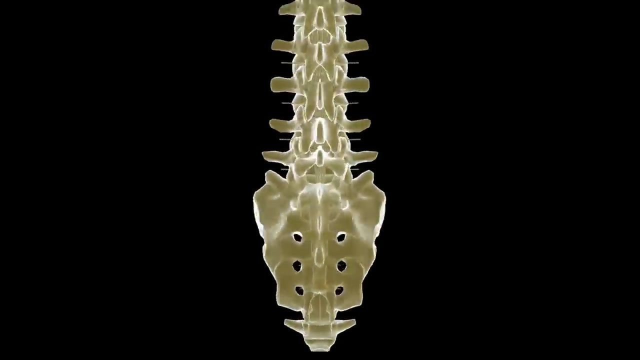 under your chest and above your stomach. The vertebrae, or spine, is made up of another type of bone called irregular bones. Jaw or mandible, and nose or nasal concha are irregular bones. So is your tailbone or sacrum. There are 33 irregular bones in your body. The vertebrae protect your spinal cord, Your spinal 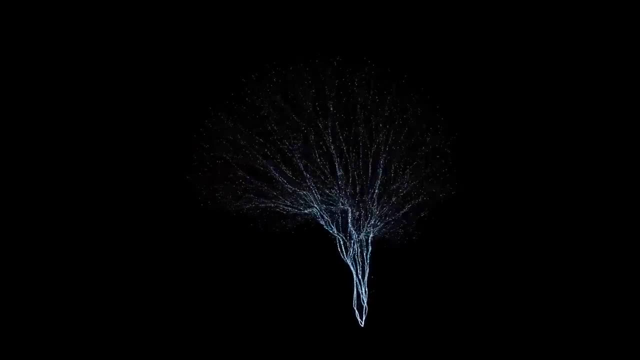 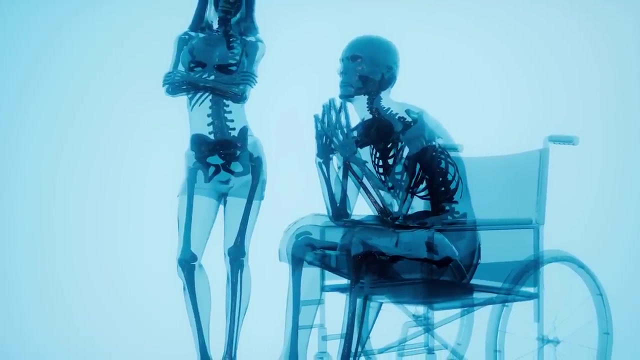 cord is the path used by the brain to send messages throughout the body. If your vertebrae was not there, your spinal cord could become injured and you might not be able to walk anymore. Sesamoid bones are bones that are made up of a lot of material. They are made up of a lot of. 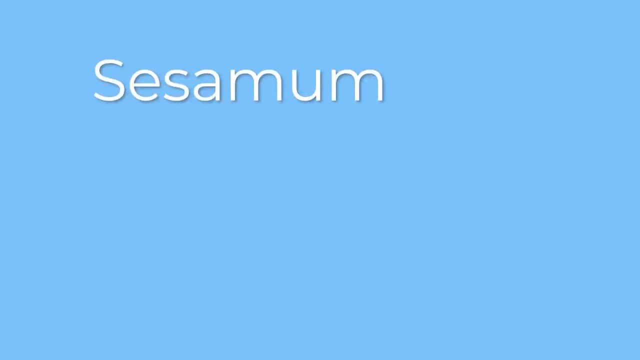 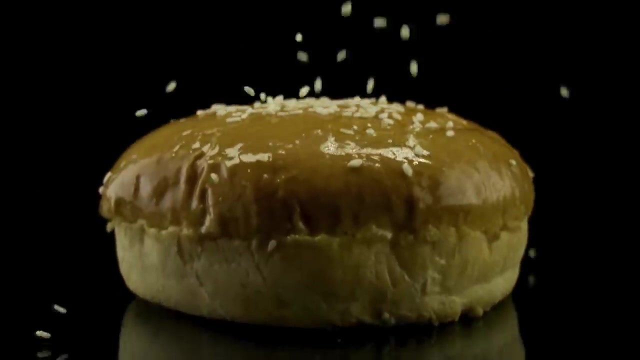 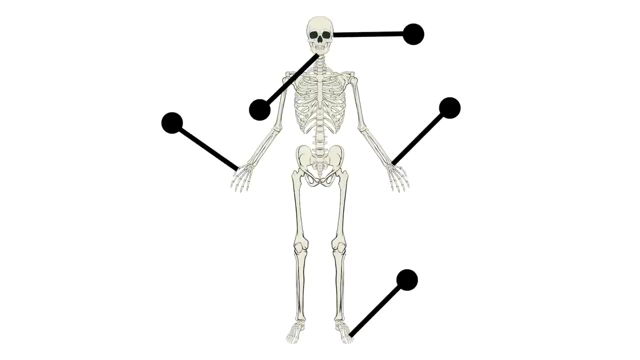 bones that are buried within muscles or tendons. The word sesamum means sesame seed in Latin. Sesamoid bones are tiny, just like sesame seeds. Some of these tiny bones are found in the hands, wrists, foot, neck and ear. The kneecap is the largest sesamoid bone in our body. 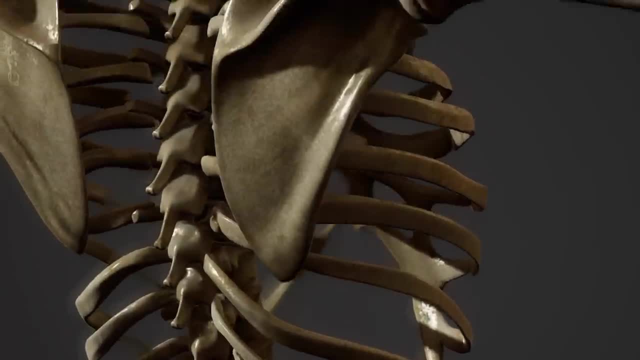 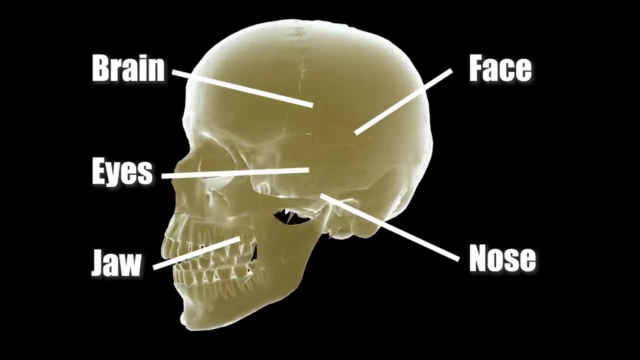 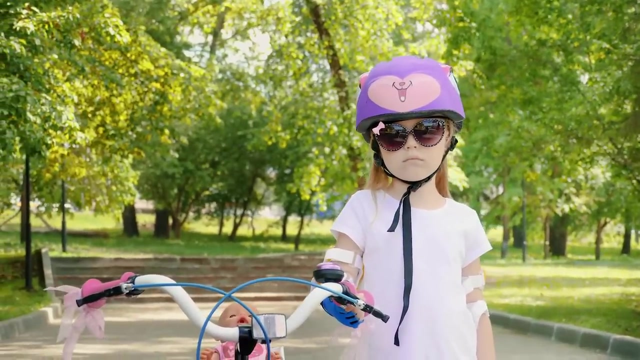 There are many different, unique and important bones in your body. Your skull protects your brain, eyes, face, jaw, nose and ears. It is important to wear a helmet when you are doing certain activities like riding a bike or a skateboard, to protect your skull. The bony ribcage covers your chest. 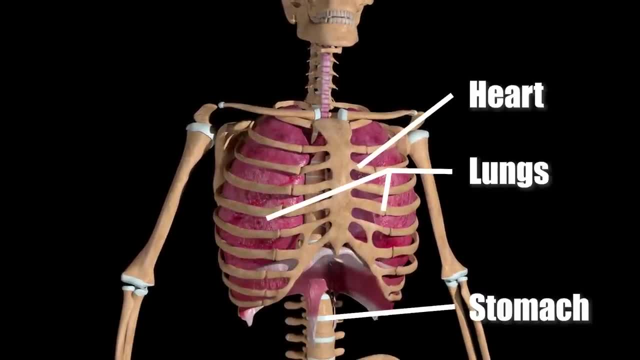 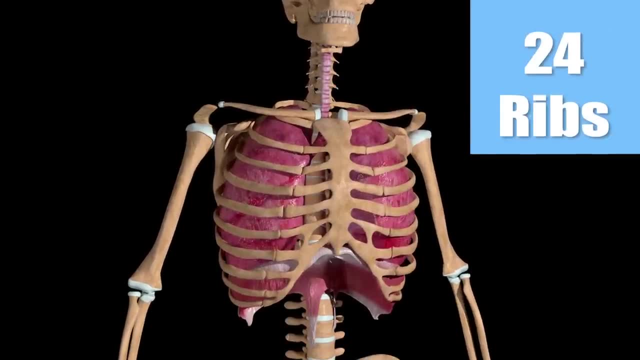 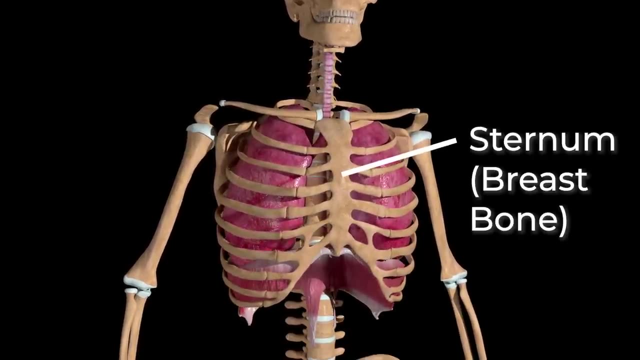 They protect the heart, lungs and stomach from injury. The typical human body has 12 ribs on each side, for 24 ribs total. Another part of the ribcage is the sternum. This part is where the heart, lungs and major blood vessels are located. It is a hard bone located in the center of the chest. 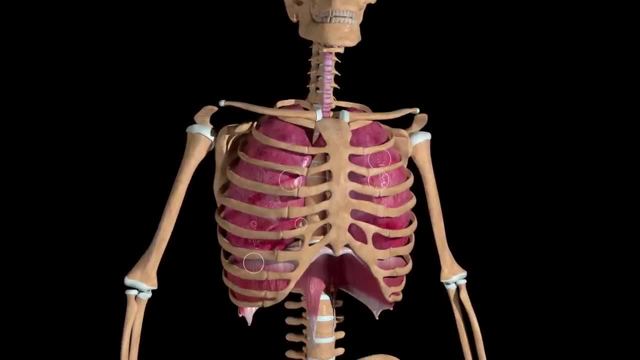 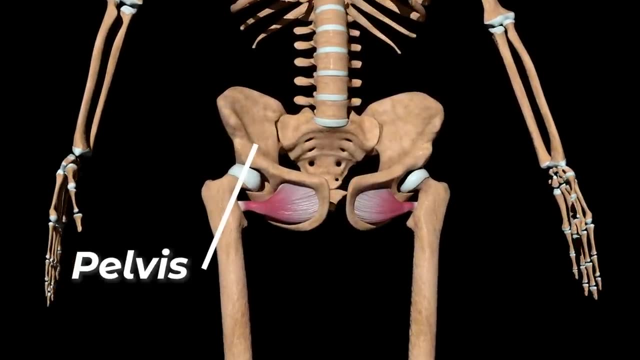 It also helps protect the heart, lungs and major blood vessels. Leg bones are attached to the bottom of the spine by a group of bones called the pelvis. The upper part of the leg is the thigh bone or femur, which runs into the knee bone. 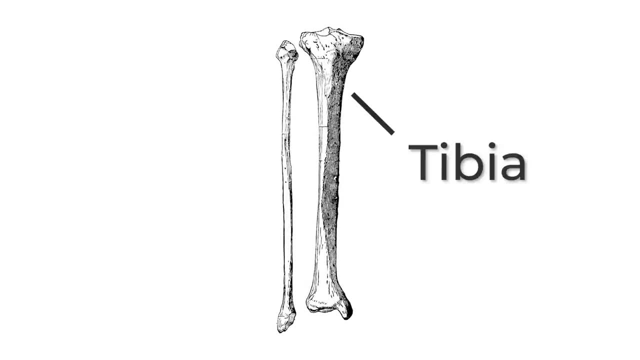 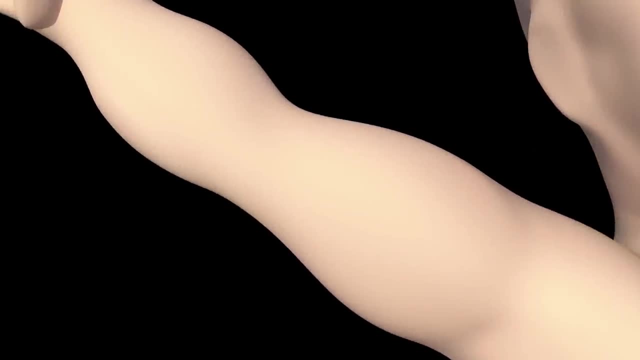 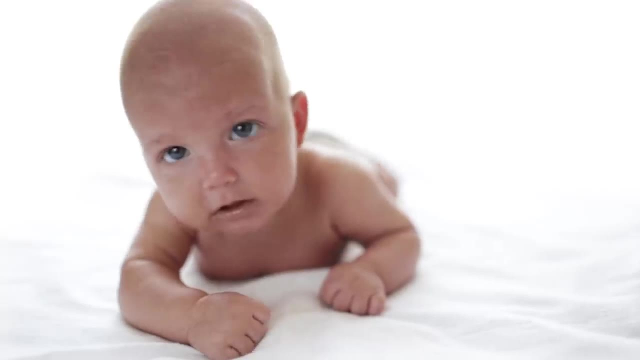 The lower leg is made up of two bones called the tibia and the fibula, which attach to the foot. The top of your arm bone is connected to your collar bone and shoulder bone. They attach to your hand. Something cool about your skeleton is that when you are born you have 300 bones. 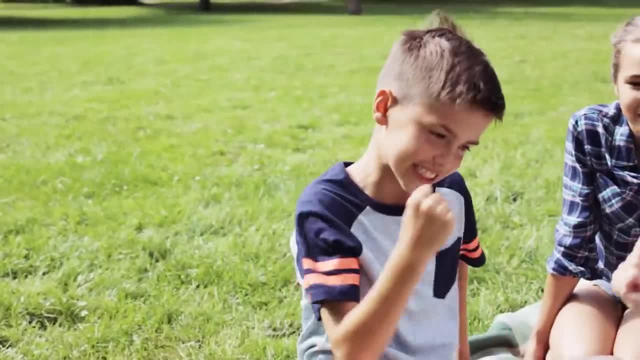 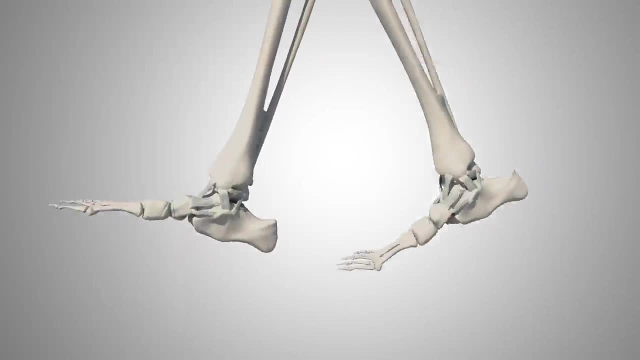 but as you grow, some of these bones join and create one bigger bone. The result is a total of 206 bones. as an adult, One fourth of those bones, or about 52 of your bones, are found in your feet and ankles alone. 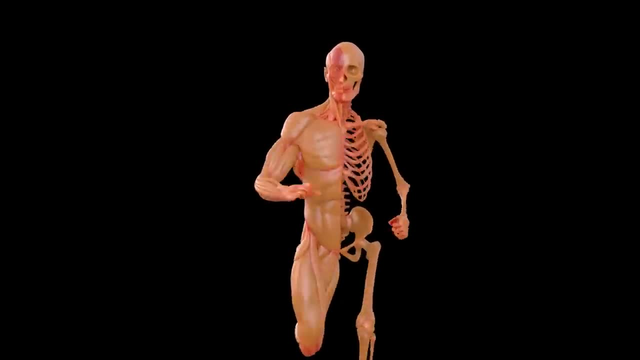 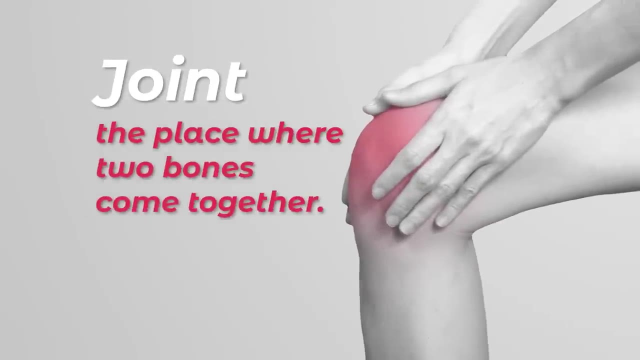 Bones work with other parts of your body, like your muscles and joints, which allow your body to move. A joint is the place where two bones come together. The knee joint is the biggest and strongest joint in the body. Ligaments then link the bones.